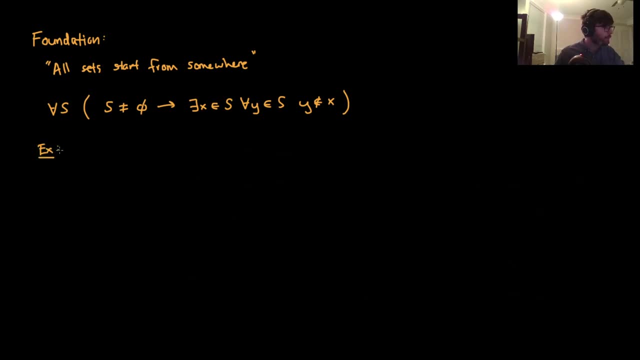 exist something like this. So here's an example: There is no set z such that z is the set containing itself. So z is a set. and one question you can ask is: well, is there a set whose only element is itself And the foundation axiom implies that there is no such set like this. So what's kind of the proof of? 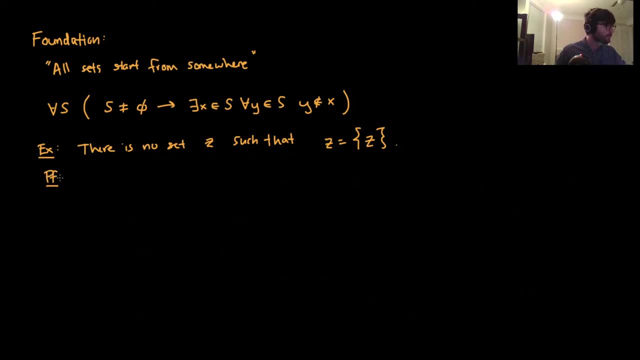 this set, or what's the proof of this? So proof, well, if there were then, well, we could, then we could apply foundation to the set z. right then, by foundation, what has to happen? Well, z is not empty. Why? Well, because it contains itself as an element. so it's. 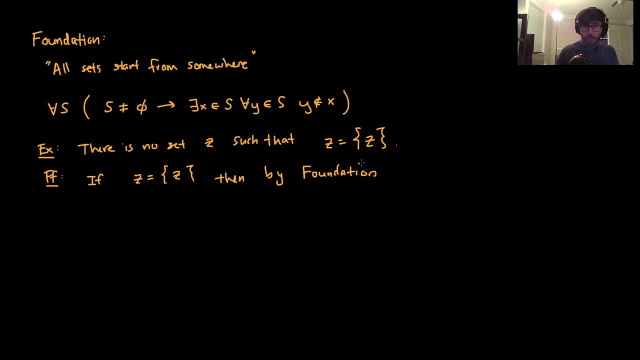 not empty. So, by foundation, there exists an x in z, so that for every y in z, y is not an element of x. That's just exactly what the conclusion of the set z is. So what does the proof of foundation tell us? Well, what has to happen? It must be that if there's a, an x and z, so that something happens. 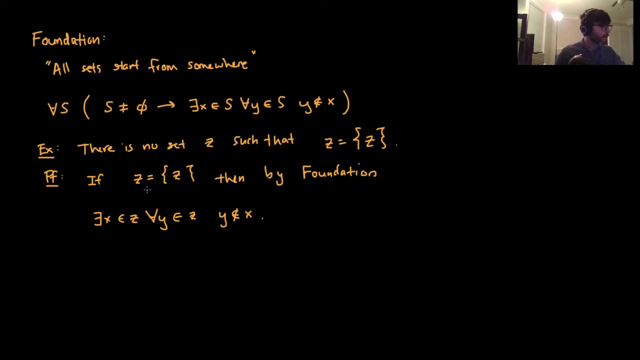 the only element of z is itself right. So since, since there's an x and z, we must have, we must have that x is equal to z. And where does the contradiction? where do we get this contradiction? Well, we have. we can pick any y for which this kind of final statement has to be true. 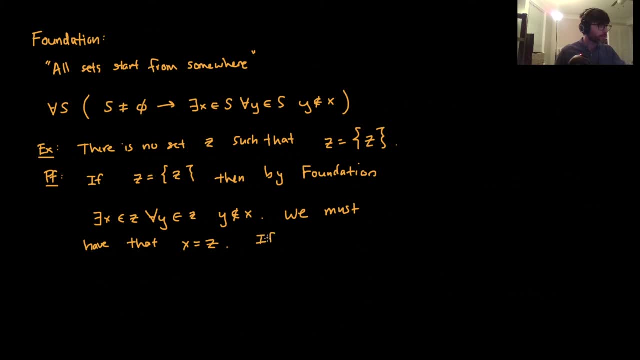 well, if y is equal to z, so if y is equal to z, then what must happen is: we must happen, it must follow that z is not an element of itself. but that's a contradiction. contradiction because, well, Z, by assumption, is an element of itself. so, by